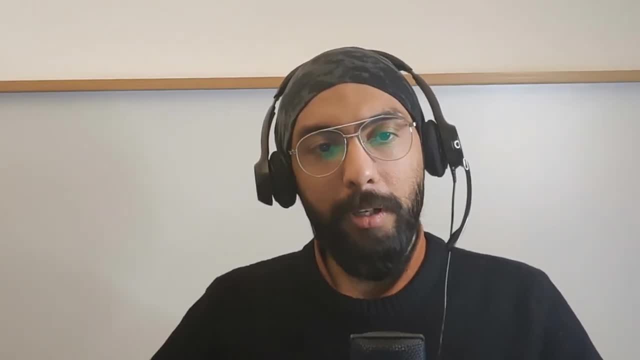 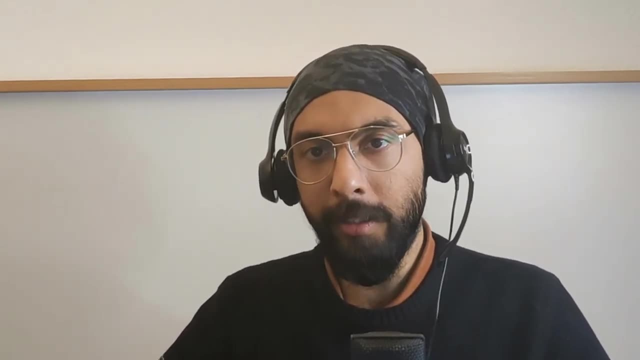 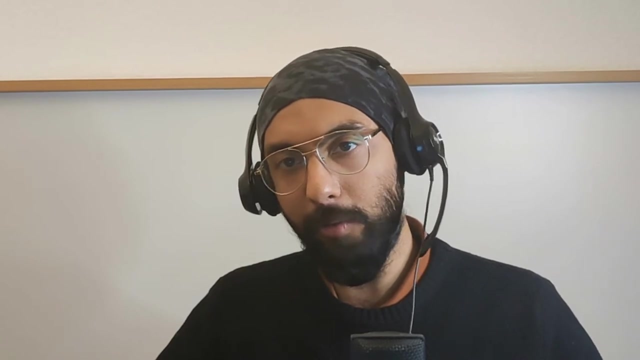 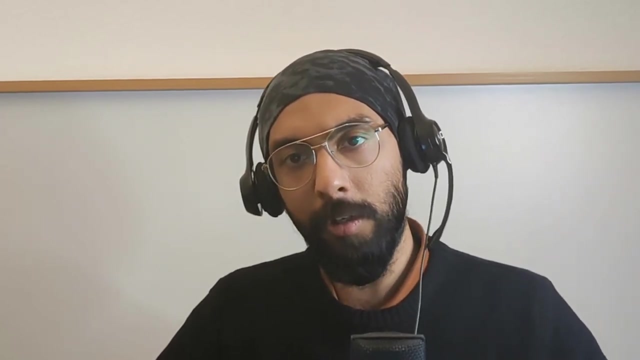 Yeah, Okay. So now let's talk about learning robotics for beginners, right? So you have been self-teaching yourself since the beginning And, of course, you took a lot of courses at the university when you did your master's thesis and all, And you worked on projects and then you worked on math works. 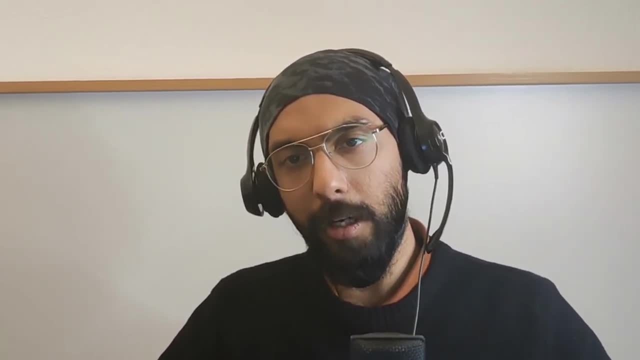 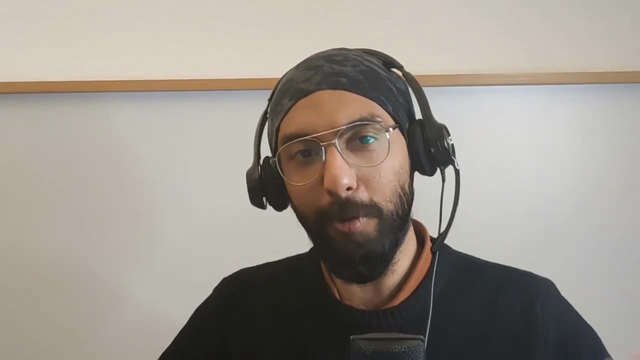 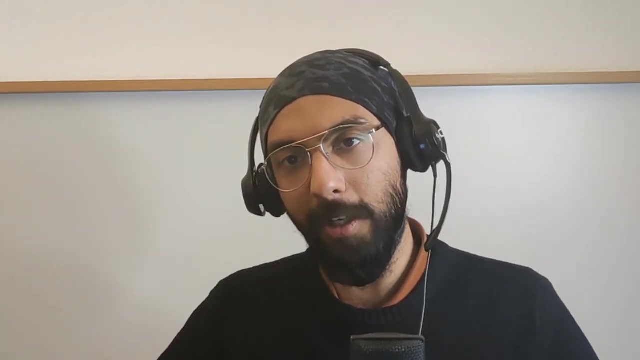 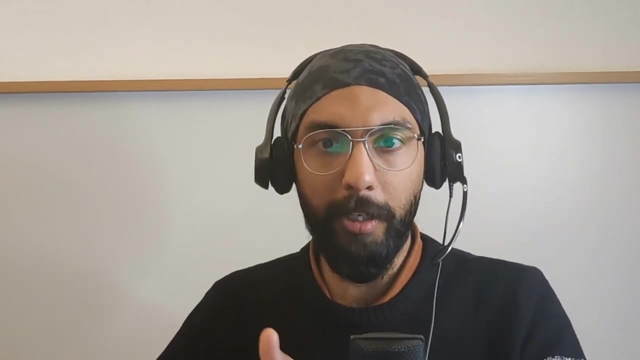 But at the same time, there's a component of self-learning involved right in all of these stages, And I'm sure you are also always self-teaching yourself, because you're also putting educational content online. So what is the best way to start learning robotics? And I think the next part would be: how do you continuously keep learning with robotics? Because you have to catch up with the research that is going on. 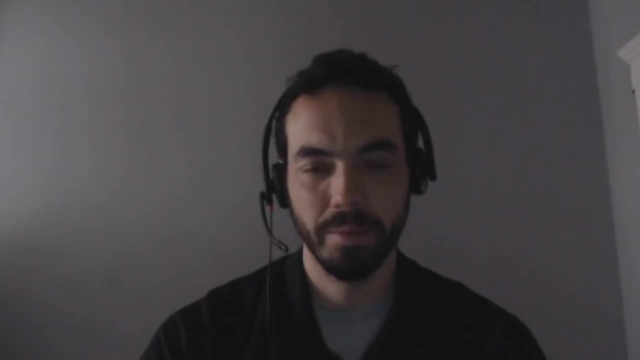 Constantly, you know, improving. Yeah, Okay, There's a lot there. I think the first thing I could say about that is that we are now in a world where it's so easy to just passively absorb information. So I will like very outright warn people to not just like watch a bunch of YouTube videos and call it a day and say that you know something. So no passive learning. 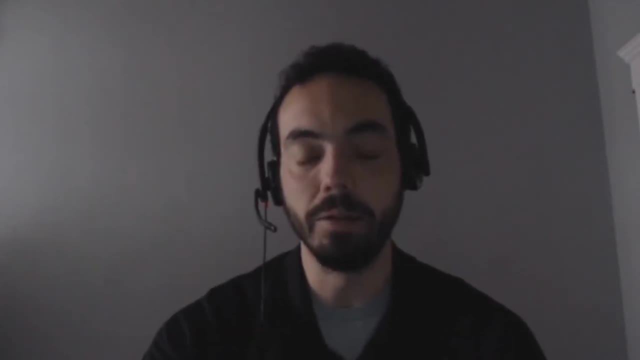 However, YouTube videos, They do have their merit And this is how I use them. I think that just watching- and by YouTube videos I mean things like you know, watching a lecture, or watching you know like a, like a lecture, a guest presentation at a university. 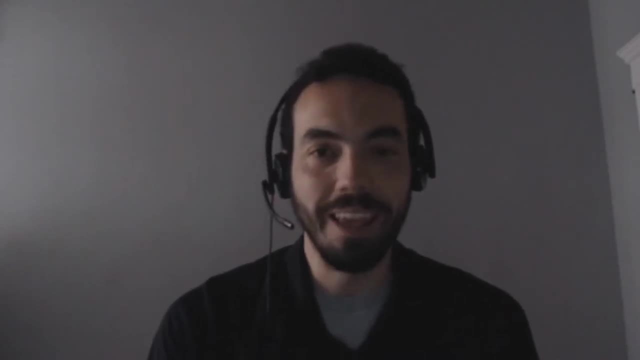 All of these things are available on YouTube now. It's great, Or like keynote speeches from conferences, that kind of stuff. I actually think it's a really good starting point in understanding the layout of the field, particularly for something like robotics, because there is just so much. 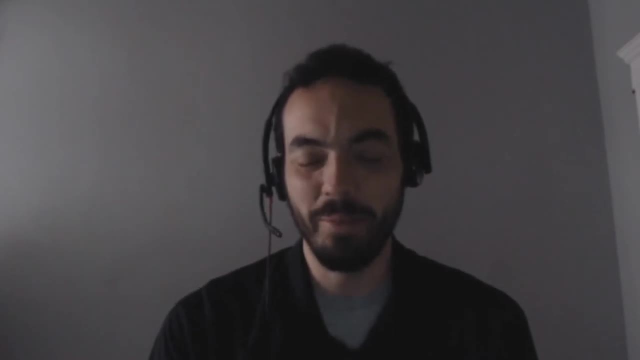 Terminology so much like jargon that whenever I'm learning a new field, like, for example, when I was teaching myself natural language processing, I just watched a couple- I spent a week watching just videos on how people talk about it, like what are all the terms that they use, like tokenization or or like, or even what are the papers that people are referencing? like you know, transformer this, transformer that nowadays. 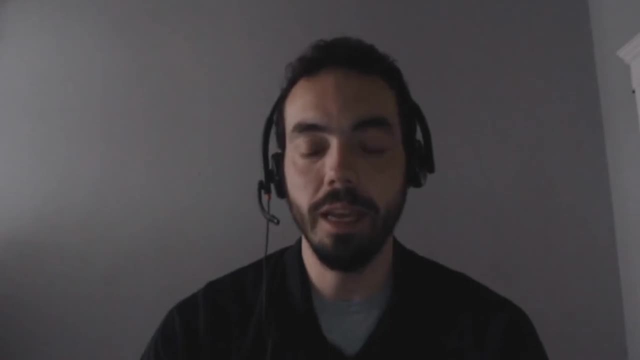 So just basically watching videos just to see how people are talking about the problems, you know what, what the state of the Art is focused on, who are the key people in the field. I think it's a good starting point so that you become kind of conversational in that area. 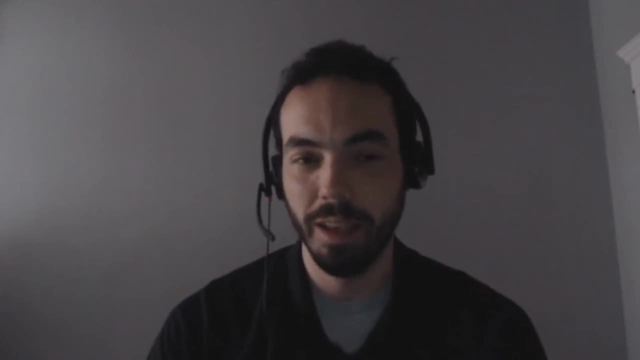 You don't yet know how to do things, but you know the purpose of things. And another example could be like: if you're trying to teach yourself computer vision, maybe you'll watch a couple of videos to understand- like What is image recognition versus classification in, versus object detection versus segmentation, like you kind of know what they're, for you don't know any of the math. 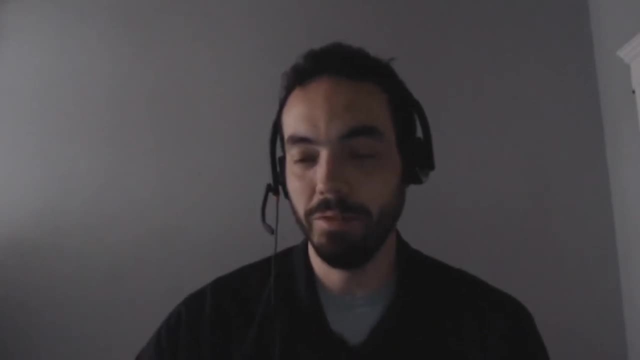 Or implementation. that's fine, OK, but you now know the types of problems, the types of solutions that exist, and that's a starting point. Then you immediately want to move on to actually doing stuff that I don't know, that I can't think. I can't think of a better way to a better alternative. 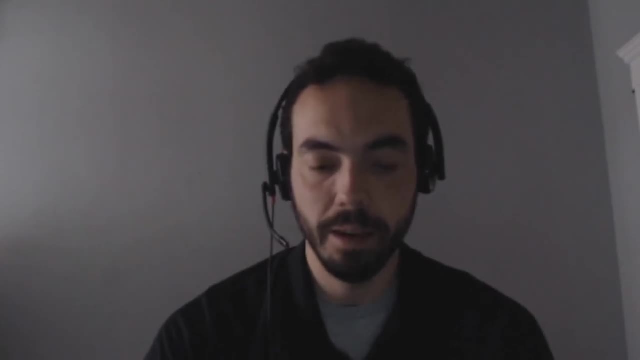 But yeah, I think actually having hands on experience is the way to go, and that can be difficult depending on how you're learning things right, You know if, if you're very self motivated, then maybe you can just open Up, like download a software package and just start like typing stuff up, or get out a pen and paper and start deriving things. 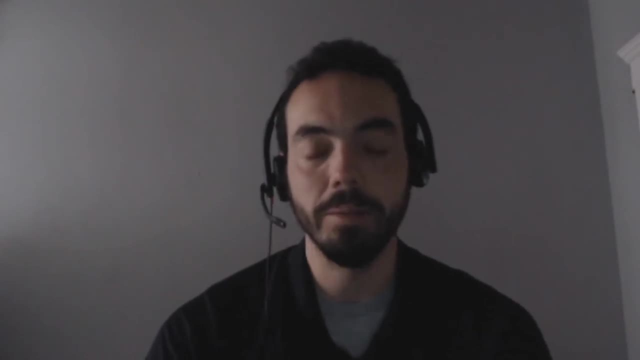 Those are all good things and if you can learn that way then that's awesome. But You know, the best way to learn something is to have a project or a problem in mind. You know, it's very different saying I'm going to teach myself TensorFlow, so I'm going to open up a tutorial and just like, run it and, like you know, change a hyper parameter, run it again, be like, oh, that's cool. 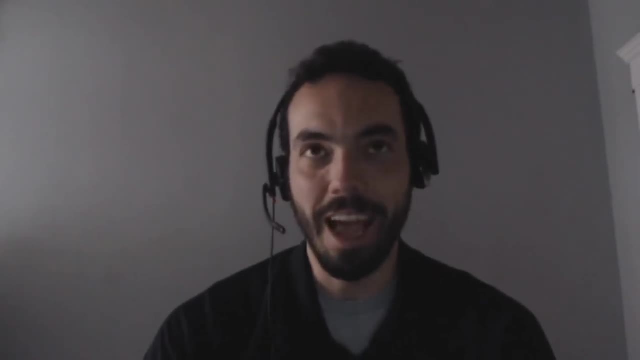 You know, learning rate helps Versus saying: I have a data set, I need to solve this problem. you know I need to classify something. What do I do? You learn a lot, because now you're not like just following along a carefully crafted tutorial. 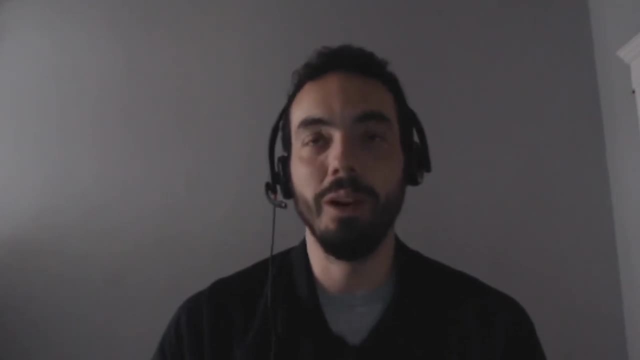 You're actually. you're actually just going to run into a lot of problems that you have to solve along the way, like: oh, maybe this network architecture doesn't work for me, You know, maybe TensorFlow was not the right tool because, you know, whatever reason, maybe I have to do something else.